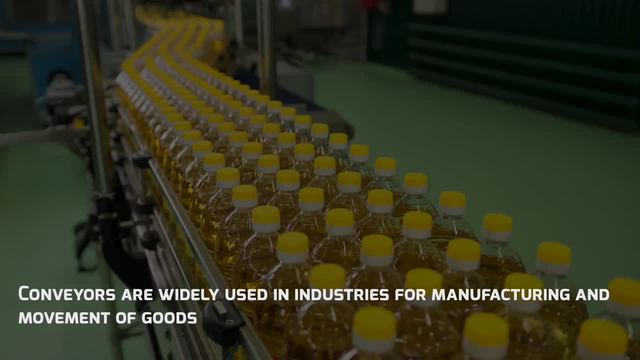 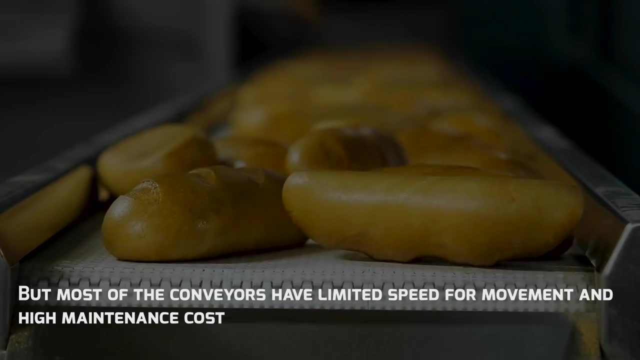 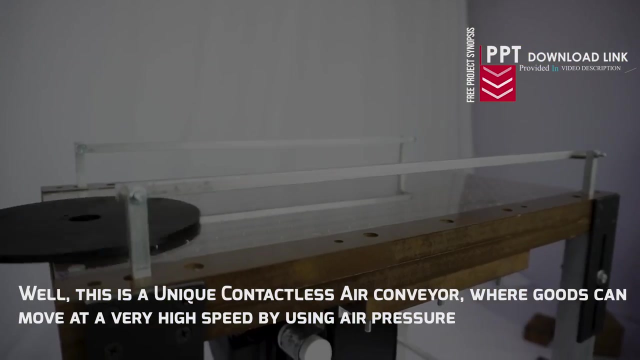 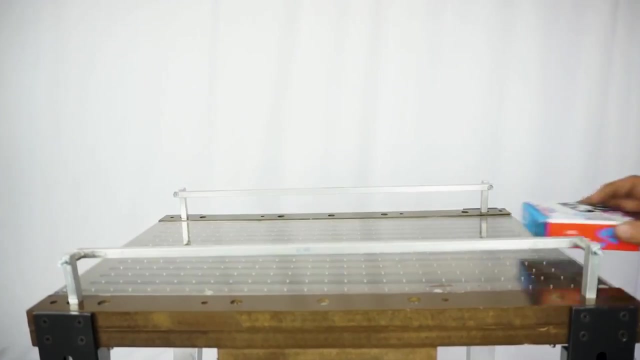 Contactless Air Conveyor Conveyors are widely used in industries for manufacturing and movement of goods, But most of the conveyors have limited speed for movement and high maintenance cost. Well, this is a unique contactless air conveyor where goods can move at very high speed by using air pressure. 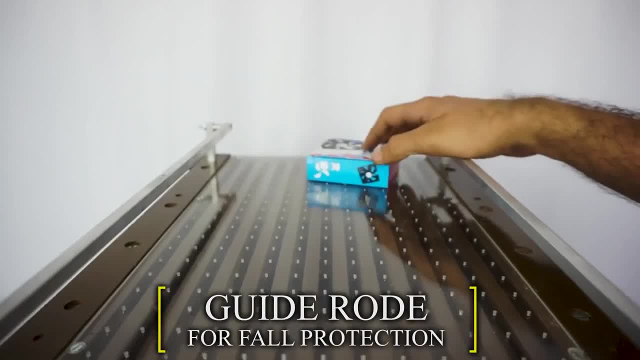 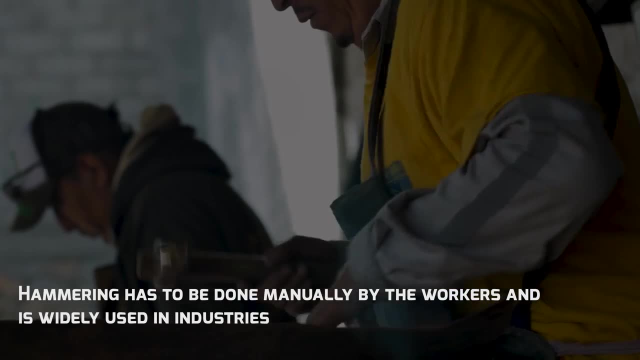 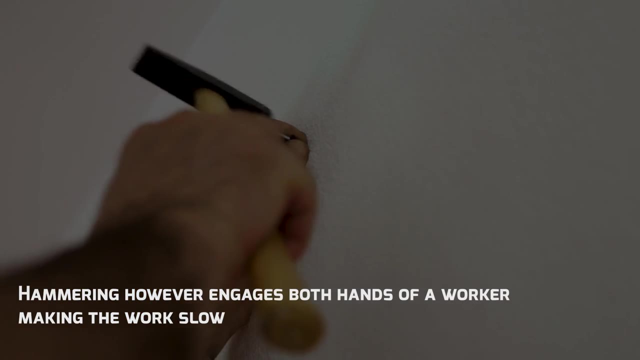 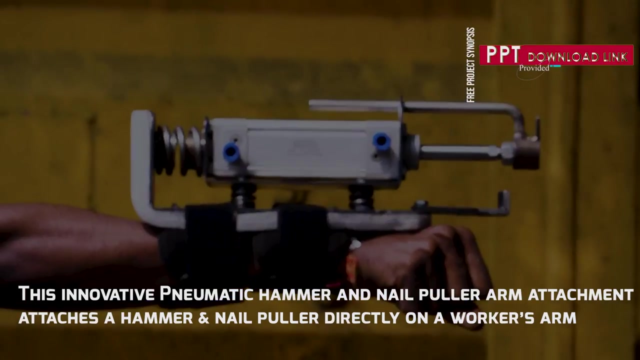 Numatic Arm Hammer and Nail Puller. Hammering has to be done manually by the workers and is widely used in the industries. Hammering, however, engages both hands of a worker, making the work slow. This innovative pneumatic hammer and nail puller arm attachment attaches a hammer and a nail puller directly on a worker's arm. 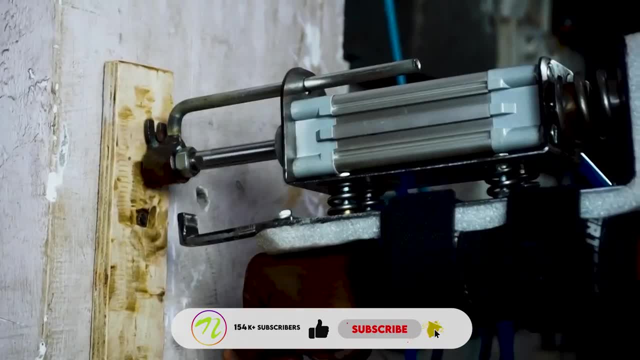 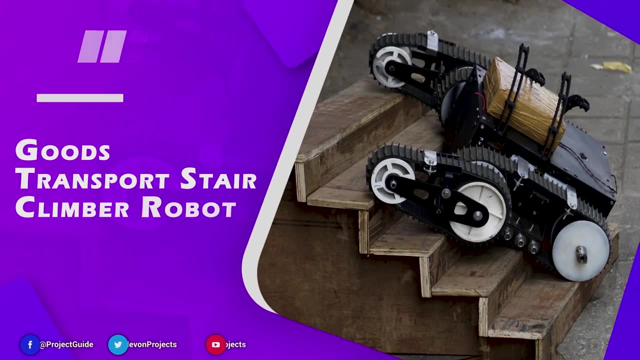 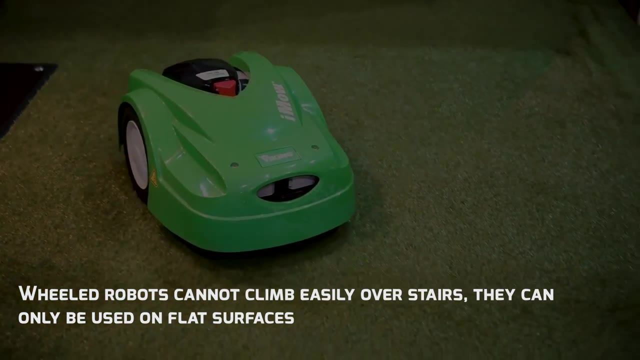 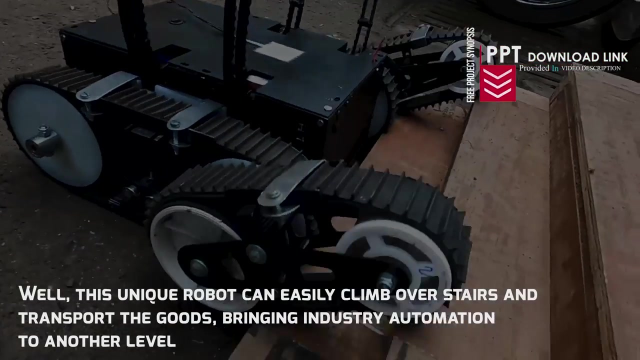 Goods Transport Stair Climber Robot. Goods Transport Stair Climber Robot. Wheel robots cannot climb easily over stairs. They can only be used on flat surfaces. Well, this unique robot can easily climb over stairs and transport the goods, bringing industrial automation to another level. 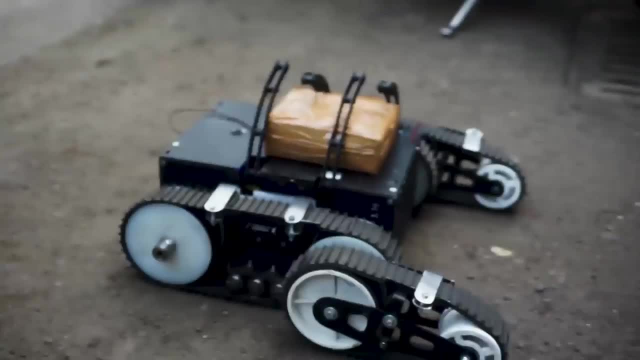 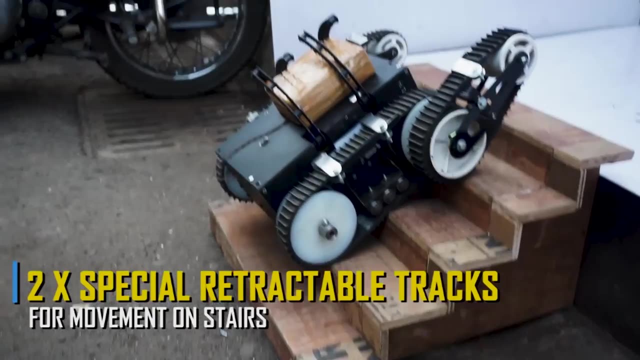 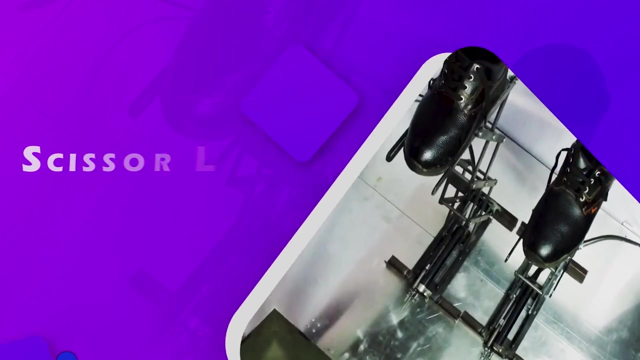 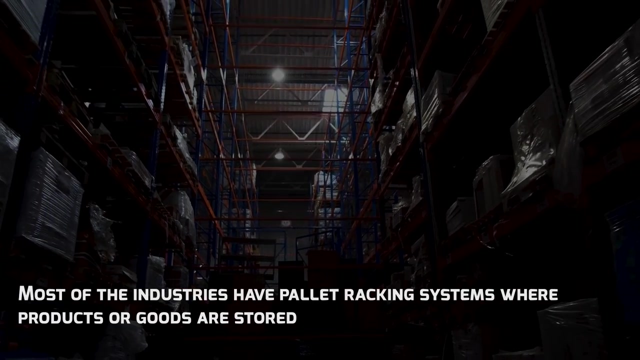 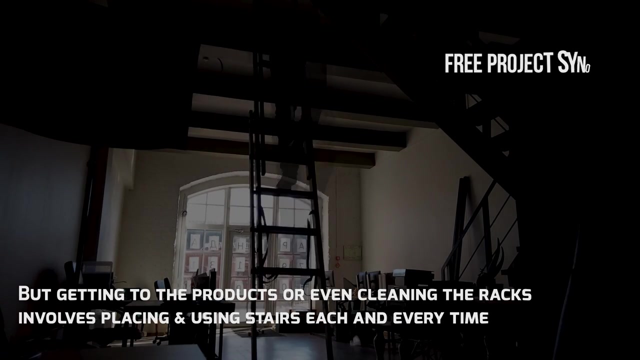 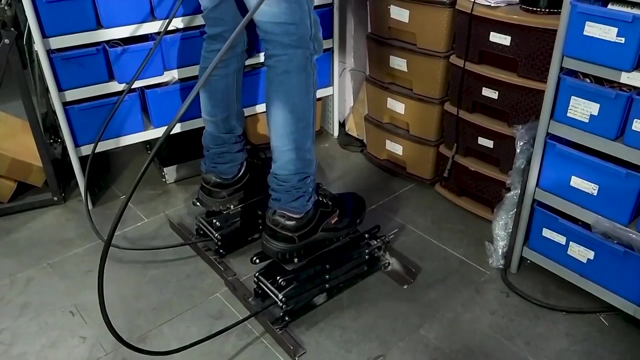 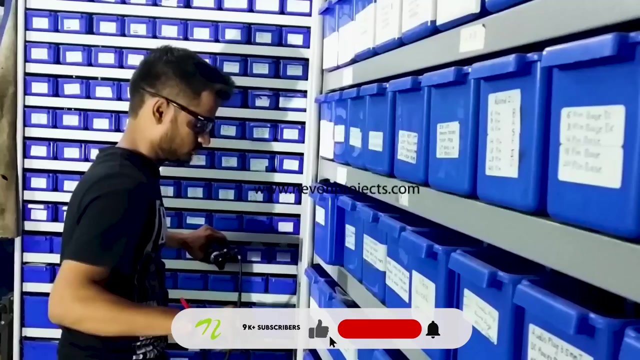 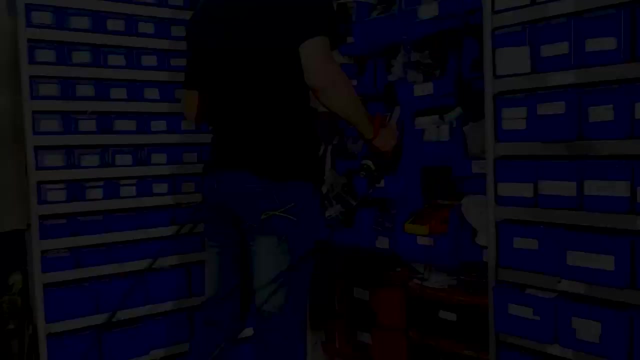 Scissor Lift Shoes. Most of the industries have pallet racking systems where products or goods are stored, But getting to the products or even cleaning the racks involves placing and using stairs each and every time. But with this unique scissor lift shoes, the workers can reach high shelves without stairs. 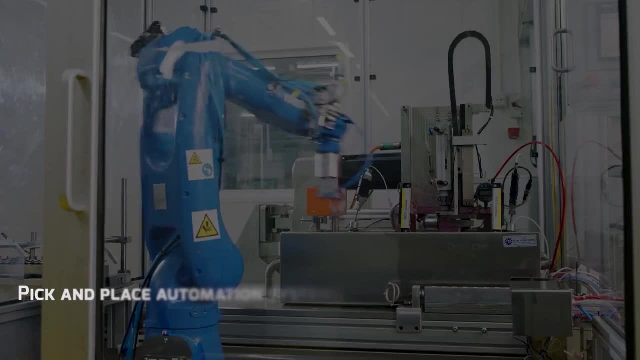 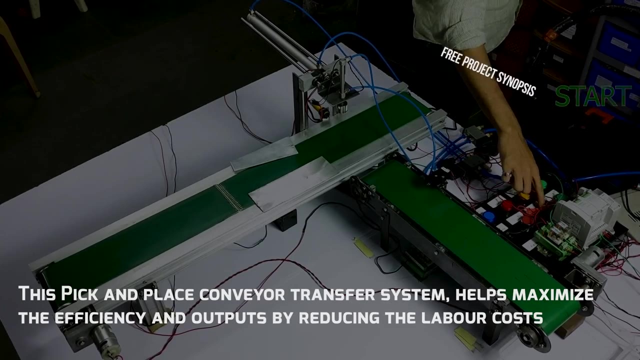 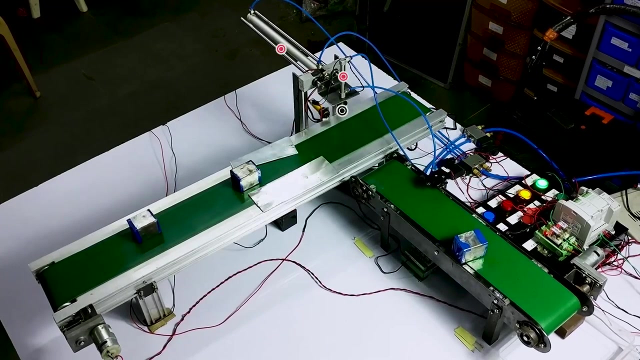 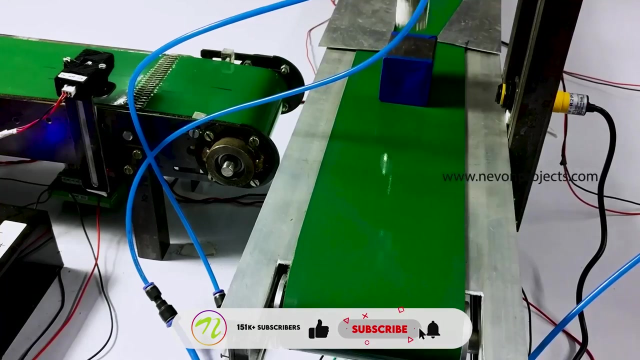 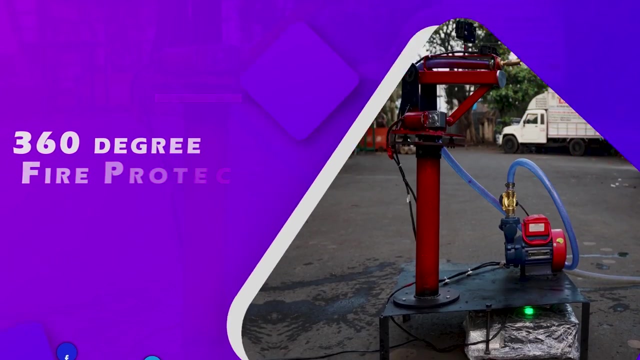 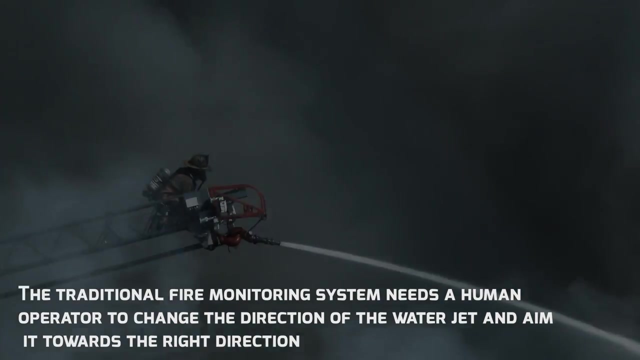 Pick and Place Conveyor Transfer System. Pick and place automation systems are widely used in industrial processes. This pick and place conveyor transfer system helps maximize the efficiency and outputs by reducing the labor cost 3-60 Degrees. The traditional fire monitoring system needs a human operator to change the direction of 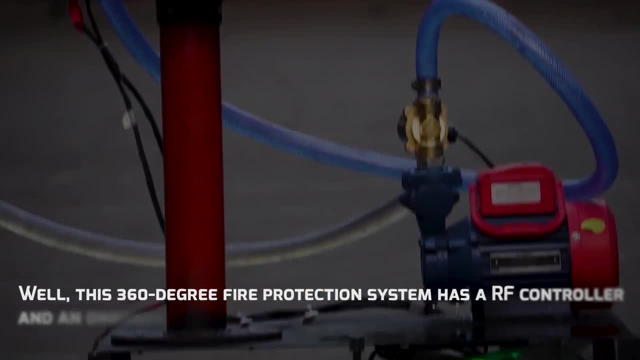 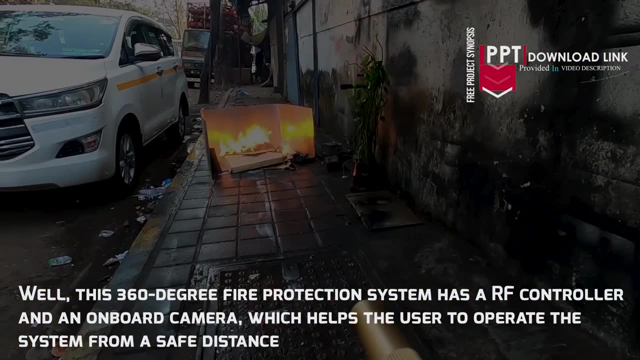 the water jet and aim it towards the right direction. Well, this 360-degree fire protection system has an RF controller and an on-board camera which helps the user to operate the system from a safe distance. 3-60 Degrees. 3-60 Degrees. 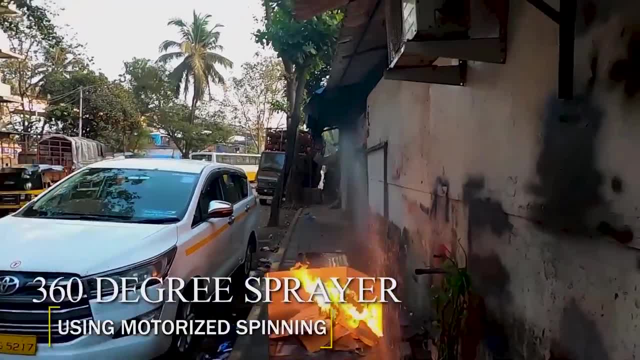 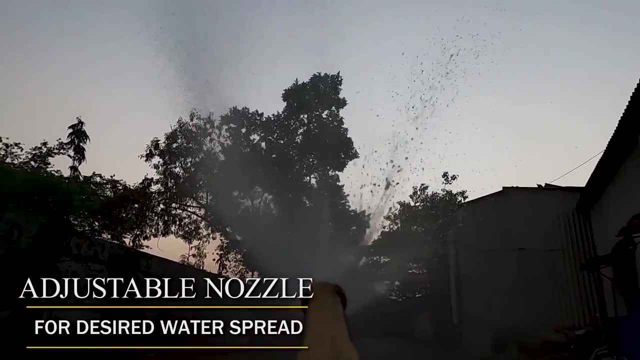 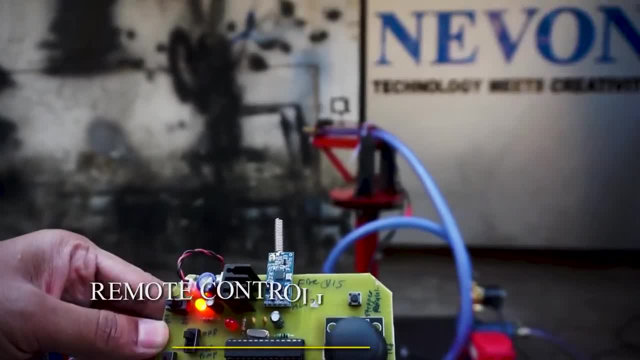 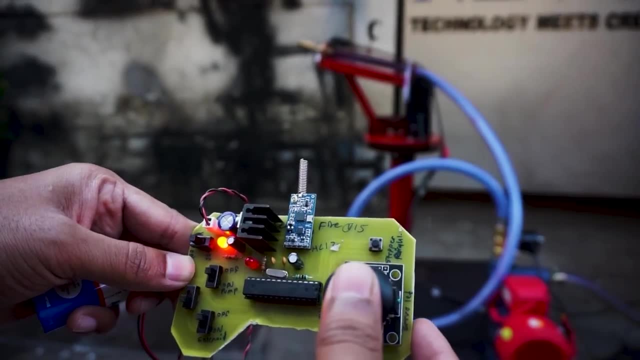 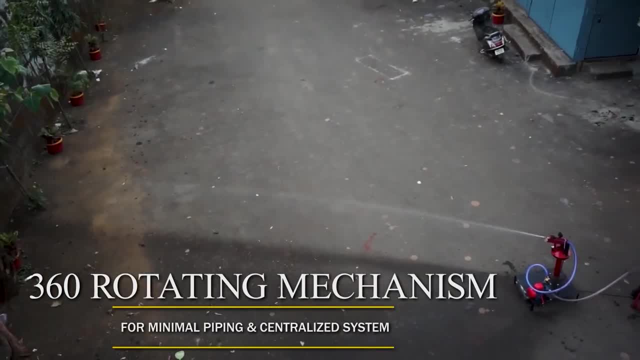 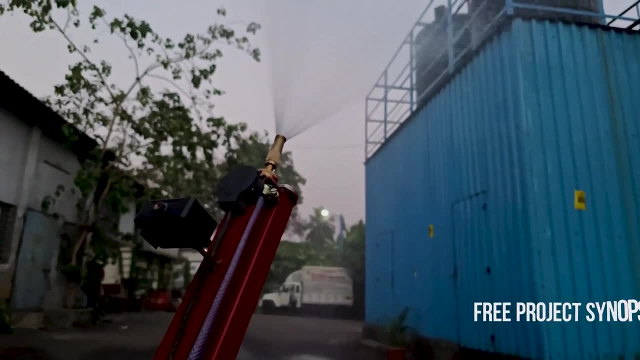 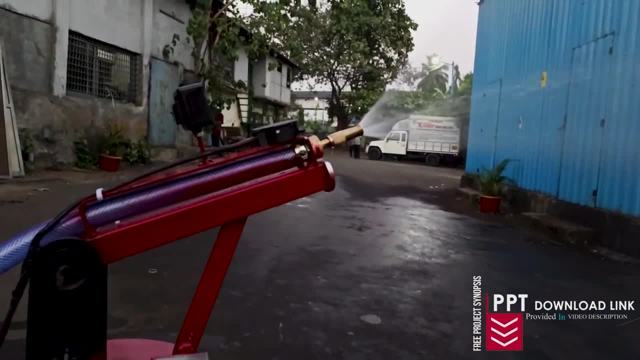 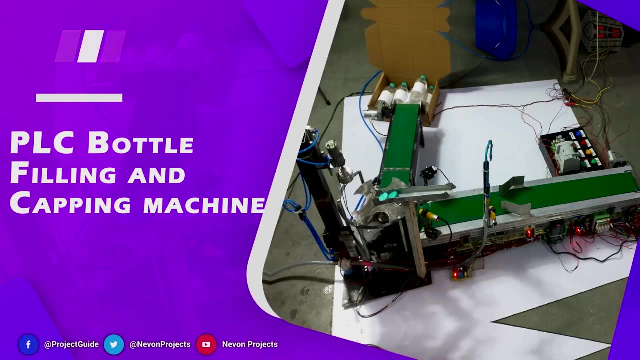 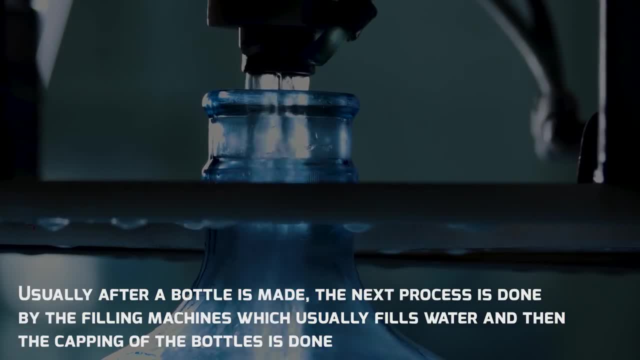 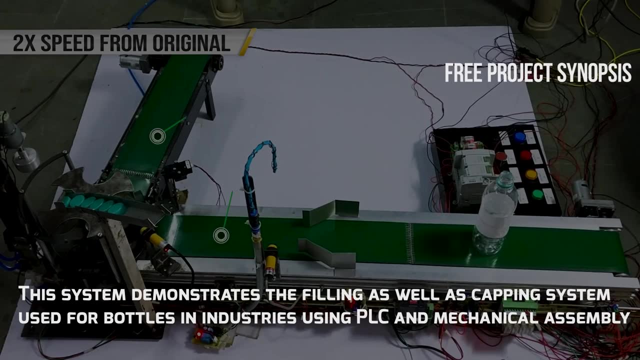 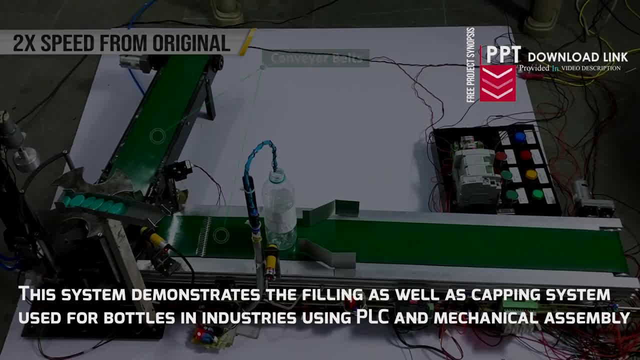 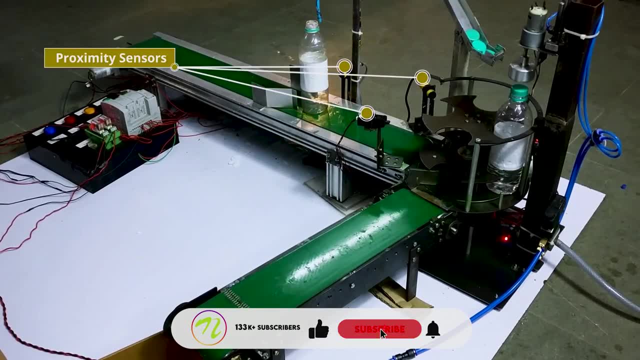 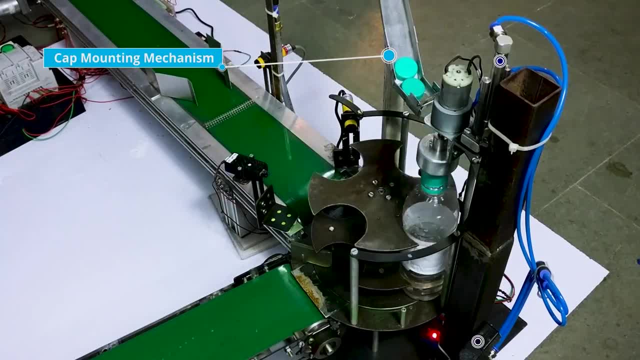 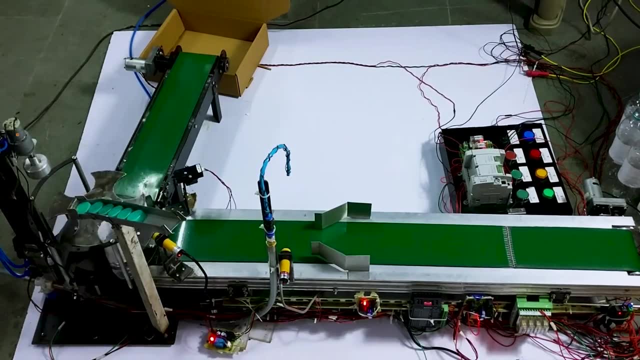 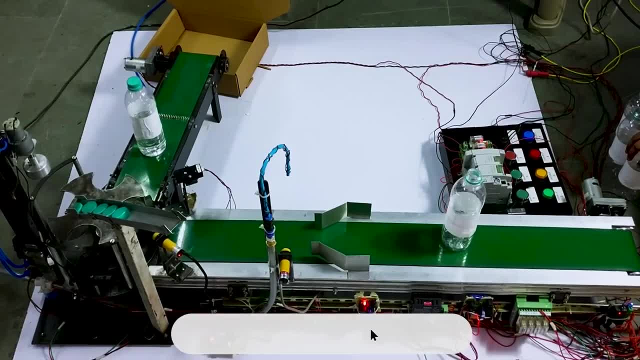 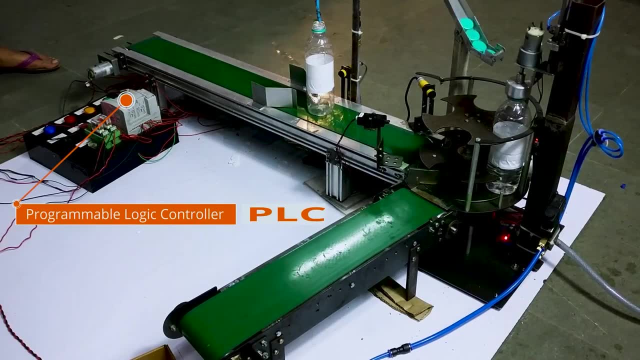 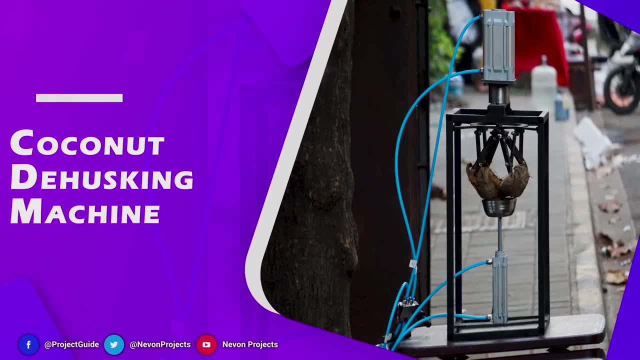 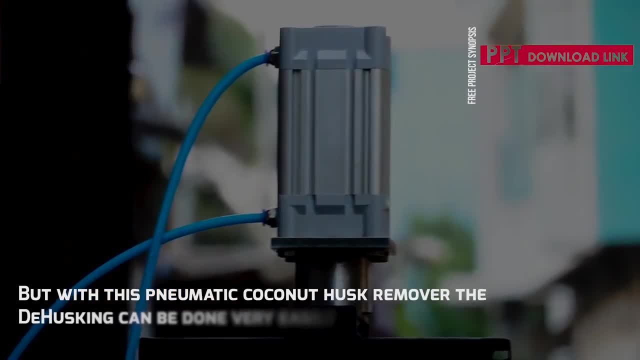